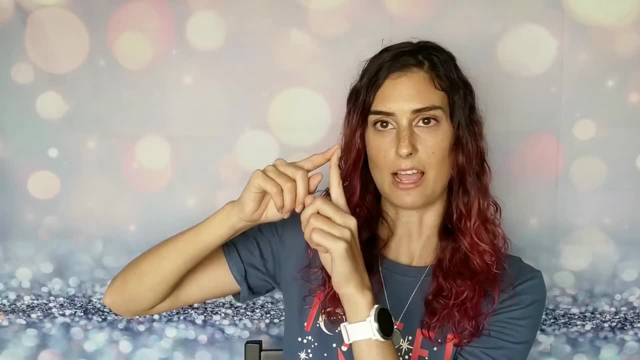 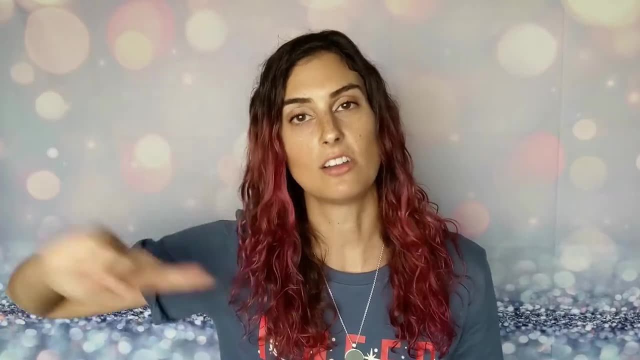 So an orientation that we typically talk about is the line of sight, which is the line between us and the thing we're observing, and then the sky plane, which is the plane that's perpendicular to it. And so radial velocity just means velocity along that line of sight. So as you can maybe 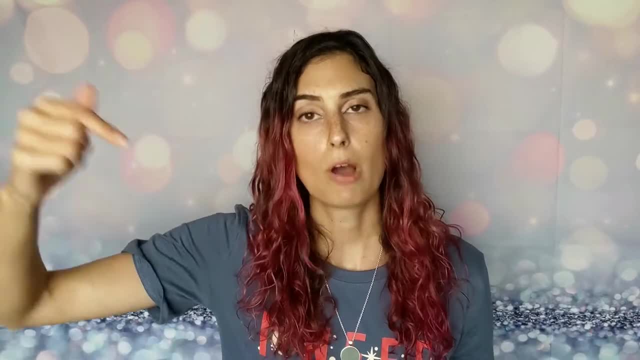 picture, as a star makes a little tiny orbit, it will have motion along that line of sight. 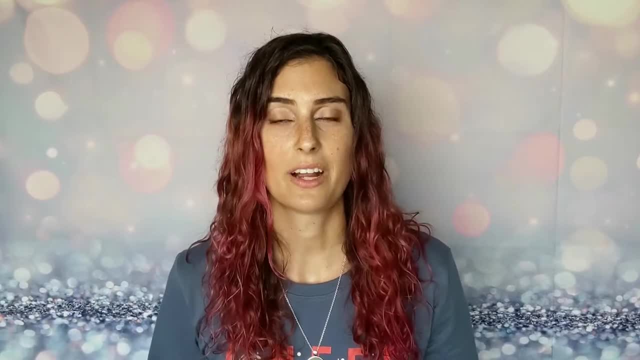 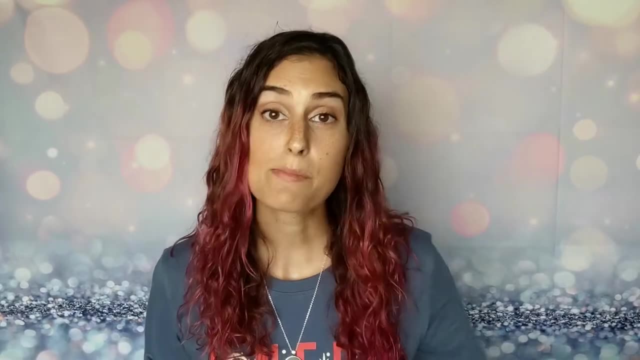 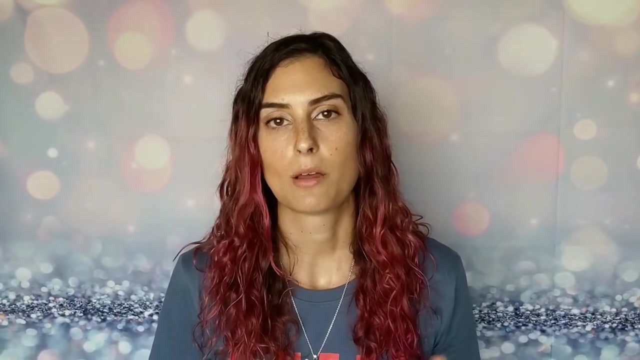 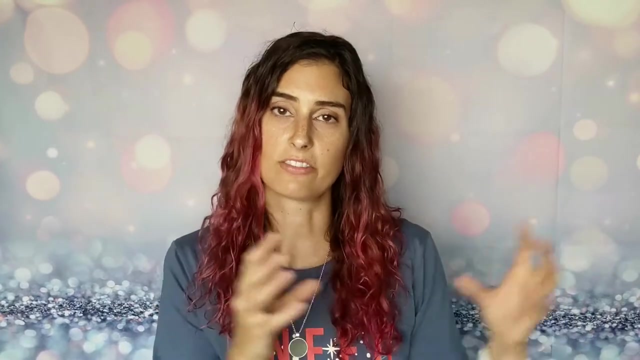 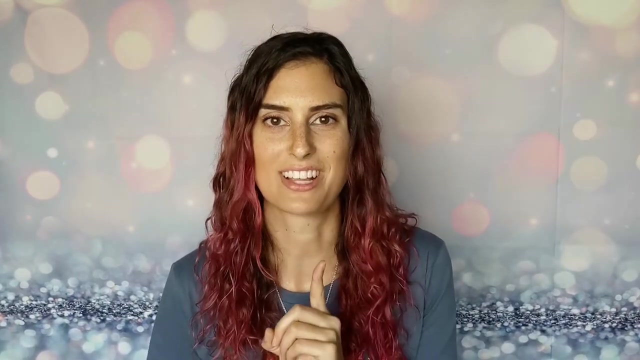 So how do we actually measure that motion? Well, this is where the Doppler effect comes in. Now you may have heard of the Doppler effect before. This is the kind of well-known phenomenon when an object comes by you and the sound changes as it comes towards you and away from you. So basically, if you have some sort of wave and either the receiver is moving or the source is moving or both, that relative velocity changes the frequency that's detected by the receiver. In this case, the receiver is moving because we are not stationary, but we can take that into account. 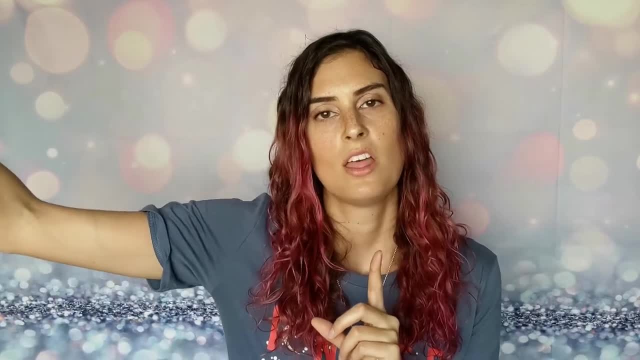 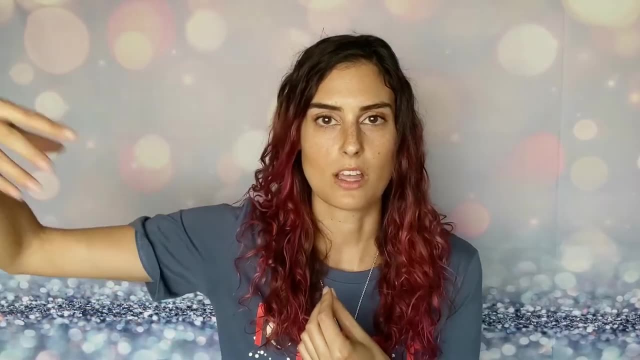 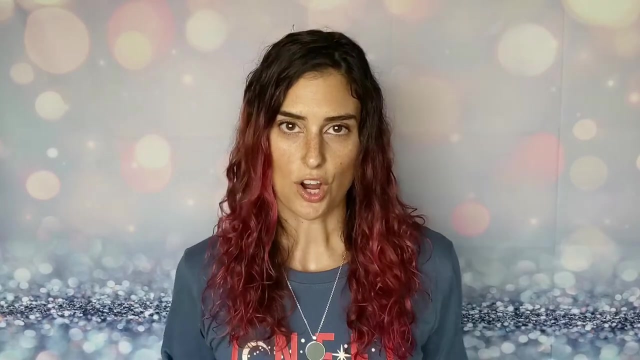 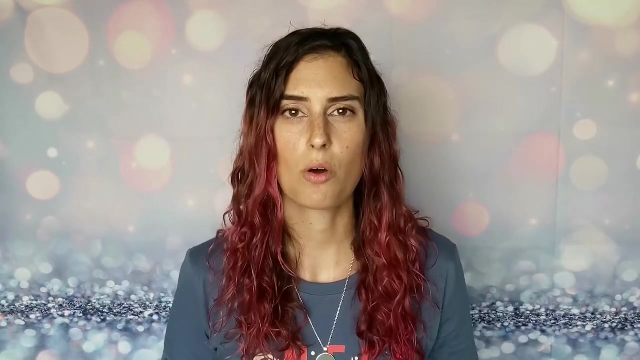 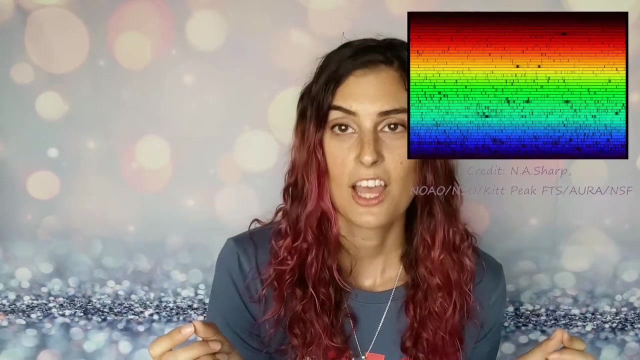 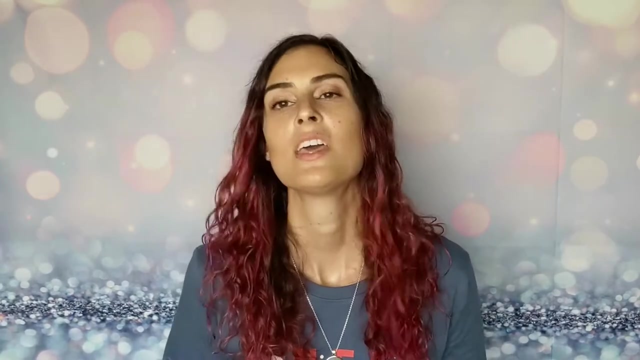 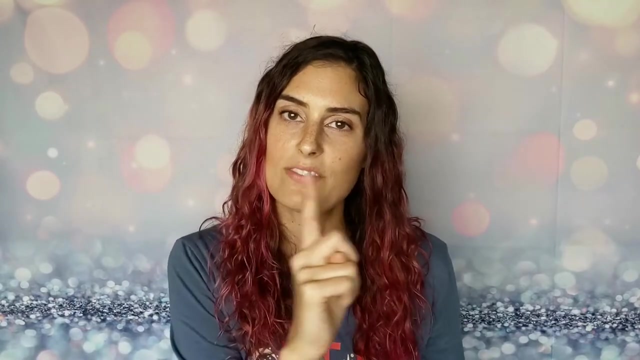 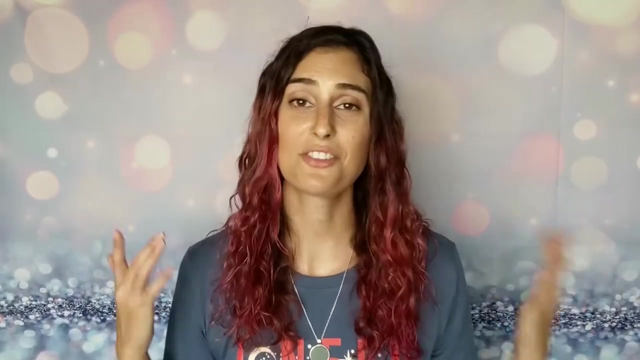 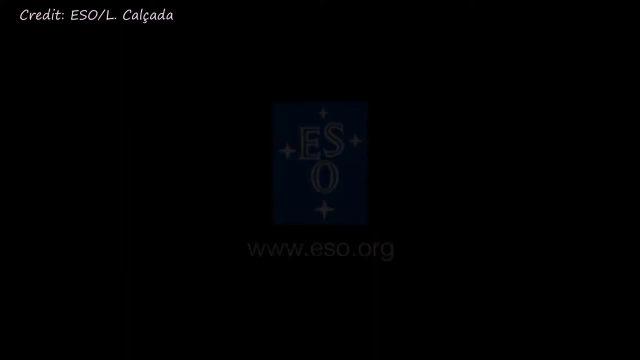 So what we're interested in is the movement of the source. And so instead of being a sound wave, like you get from an ambulance, in this case it would be a light, wave. And so as the light from the star comes towards and away from us along the line of sight, it is Doppler shifted. And the way we measure that is because every star has very particular spectra, and it has lines in the spectra. So for example, if you broke apart a sunbeam in a prism, it looks like a rainbow. But if you look at it really, really closely, you will see that there are little absorption lines where the rainbow doesn't come through. And those happen at very specific wavelengths that we don't see. So if you look at a sunbeam in a prism, it looks like a rainbow. And so it's a measure of how fast the stars are moving towards and away from us. So you can see those wavelengths in a star, and then as the star moves towards and away from you, those wavelengths will actually shift back and forth. So we can measure that shift, and that tells us how fast the star is moving towards and away from us. And so this gives us information about the star's motion, which we can then use to infer things about the planets that are around that star. And so here is a nice little illustration of what this kind of looks like, if you're having trouble picturing this, which I wouldn't blame you if you would, because there's a lot of different pieces that go in and out. So if we can take a second look at our star, we can then a little illustration of what it looks like. But again, we can measure the shift, and that tells 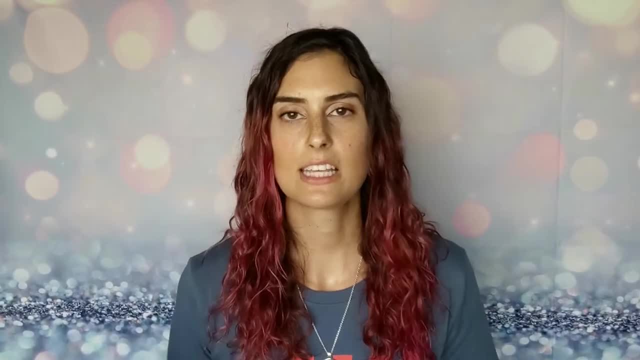 that go into this. So just as in timing, since in this case we're detecting the motion of the star along the line of sight, we're getting 2D information about the orbit, not 3D information. 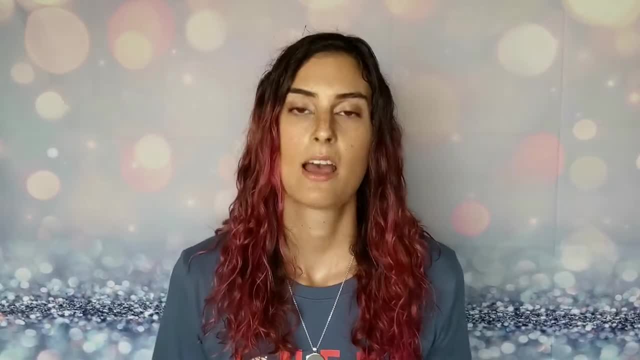 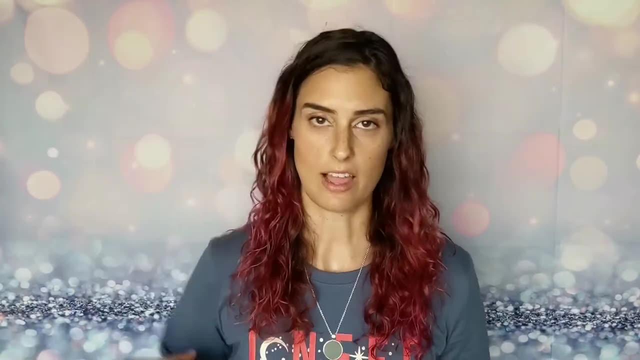 And so we can get a mass from this, but it's only a minimum mass, or an m sine i, because there's a degeneracy between the mass of the planet and the inclination of the planet's orbit to the line of sight. So if we're observing it directly edge on, then we are getting the actual mass, but if it's 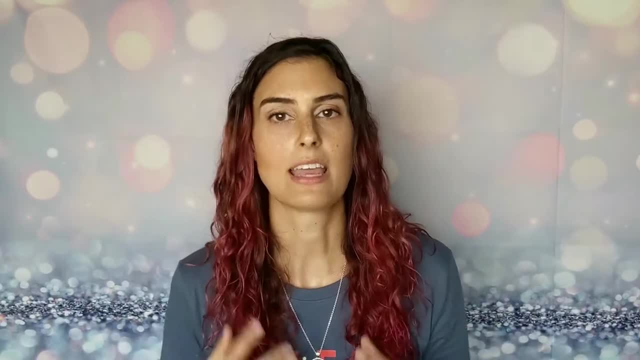 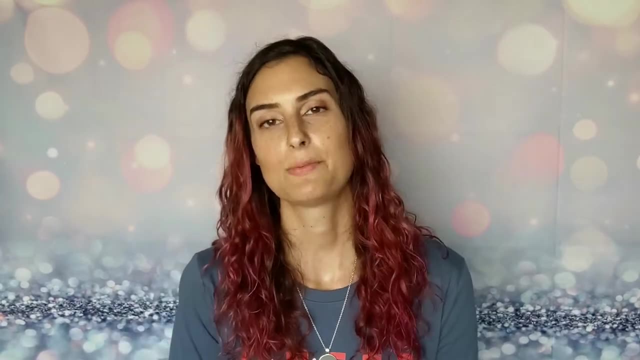 even slightly off, we're getting just a slightly lower mass than the actual planet has. So one thing that's great about radial velocities is that we do get masses, which you don't necessarily get from some other methods, and especially when combined with other techniques that can be really 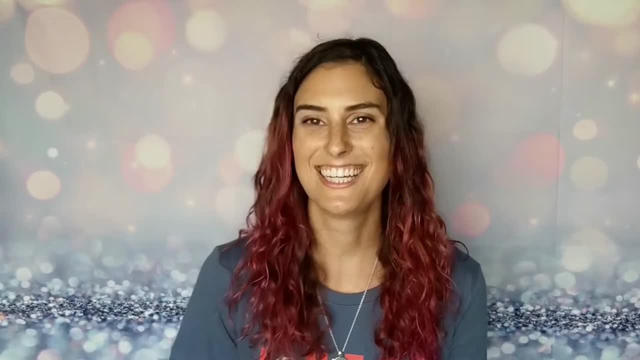 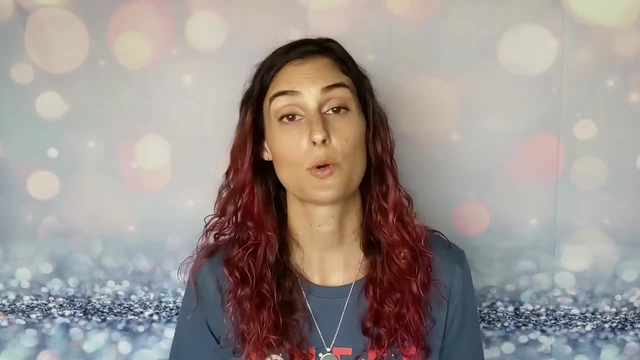 powerful, and we'll talk more about that when we talk about trademarks. But a disadvantage of radial velocities is that you have to contend with a lot of noise from the star. So a star has spots, 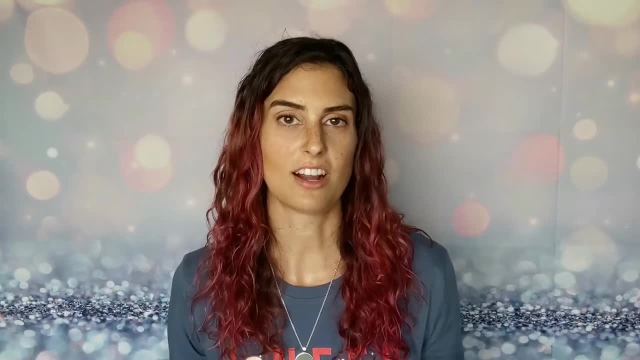 it rotates, it has flares, there's a lot of things going on with the star, and so this very kind of simple picture that I'm showing you right now is a very simple picture of a star, and it's a I've painted can become very complicated, especially because the type of signal that 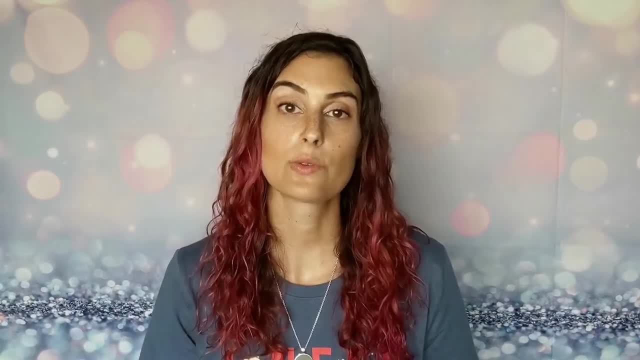 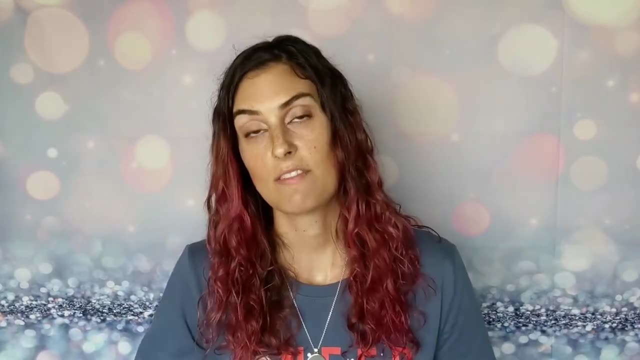 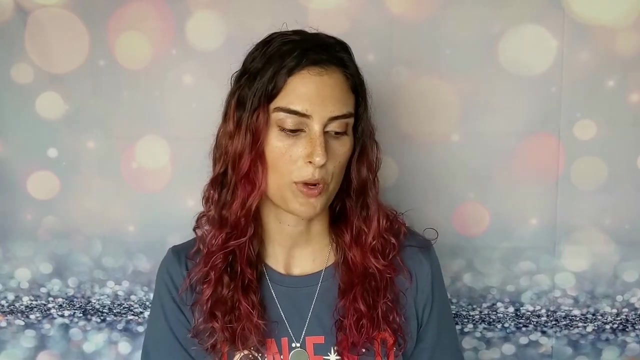 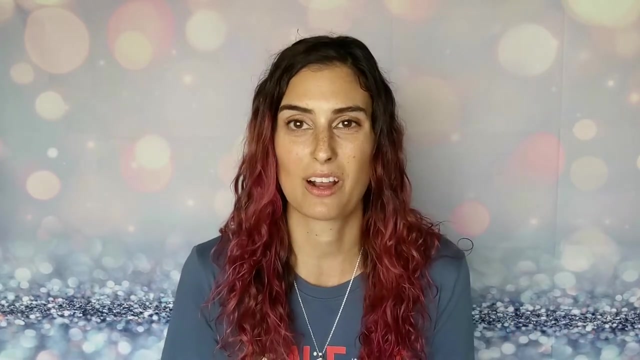 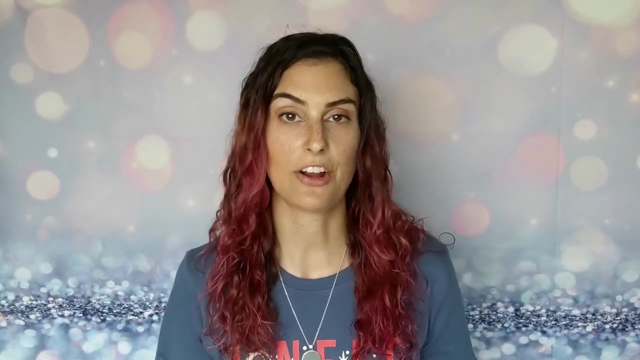 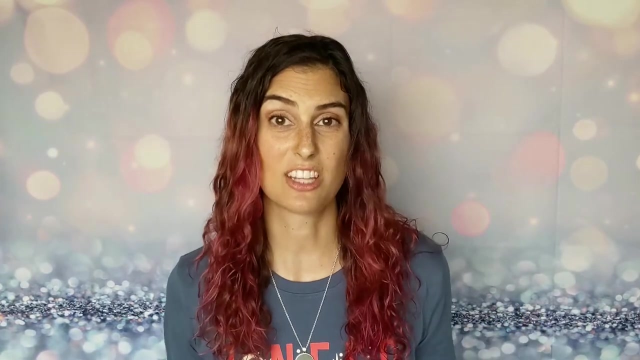 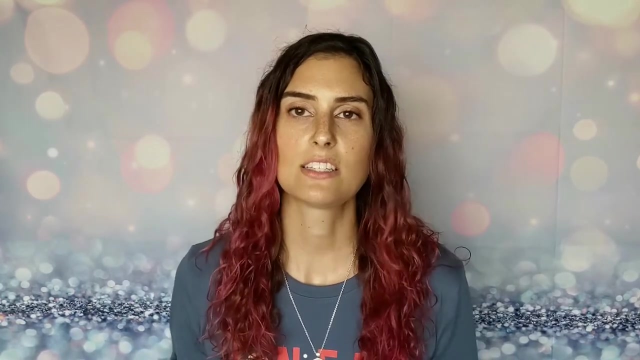 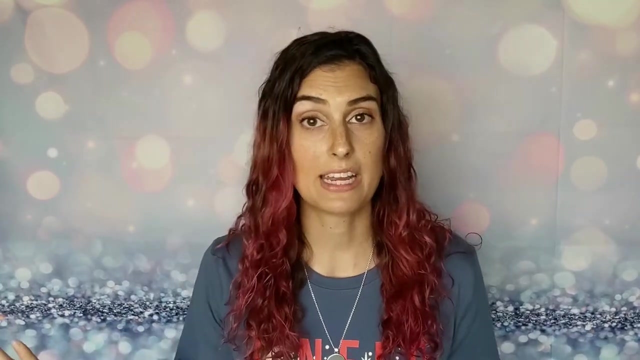 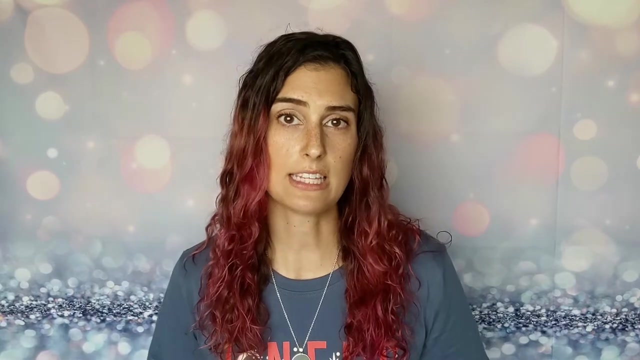 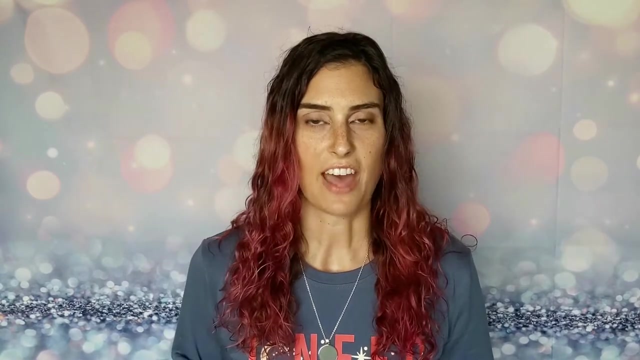 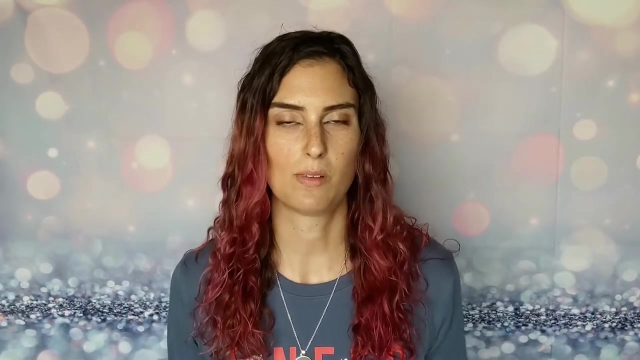 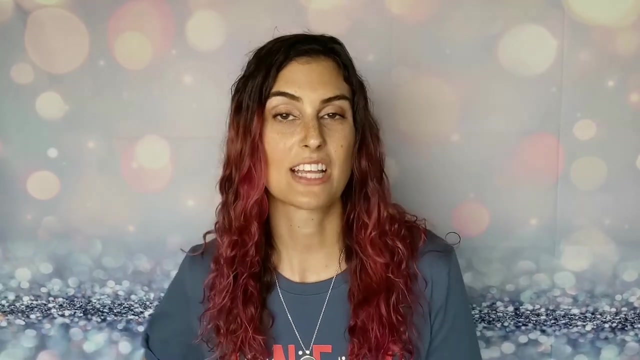 we're looking for is actually really, really small. This signal is normally called the radial velocity semi-amplitude. It depends on the period, mass, and inclination, and eccentricity of the planet, as well as the mass of the star. And so for example, our own Earth around our sun would have a signal of about 10 centimeters per second, which is very, very small compared to all of this other noise and stuff that is going on in a spectrum. However, this has been a really active area of instrumentation research, and instruments are getting very, very precise. There's a new generation of spectrographs that can actually get down to this sort of 10 centimeter per second accuracy. And one thing that has been kind of a trend is to look at smaller stars in the sun, because like I said, the signal depends on the star's mass. So as the star's mass gets lower, the signal from the planet gets stronger because the star gets pulled around, more by the planet. And so a lot of radial velocity surveys are now targeting what we call m-dwarfs, which are the smallest kind of stars out there. And another advantage of that is that if you're interested in planets that are in the habitable zone, which we can talk about in another video, but basically this is planets that could potentially have life, like the Earth, the habitable zone for an m-dwarf is actually much closer in, so you'd be looking for closer in 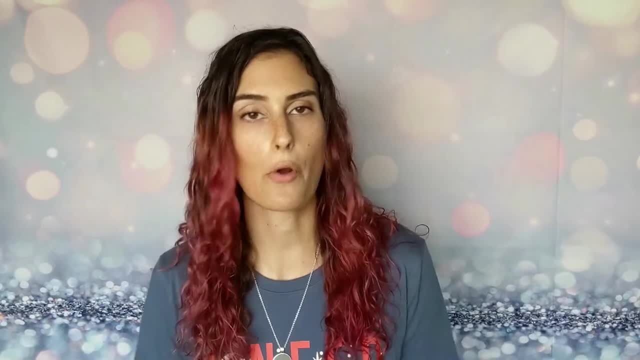 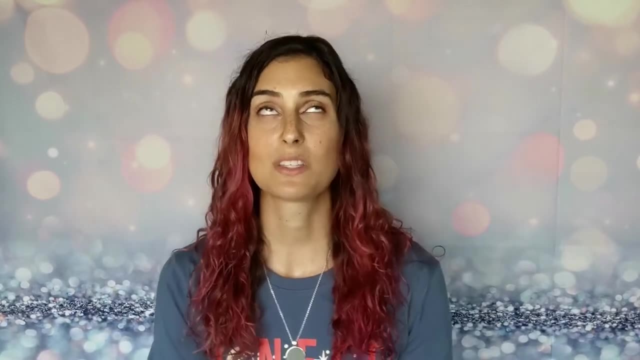 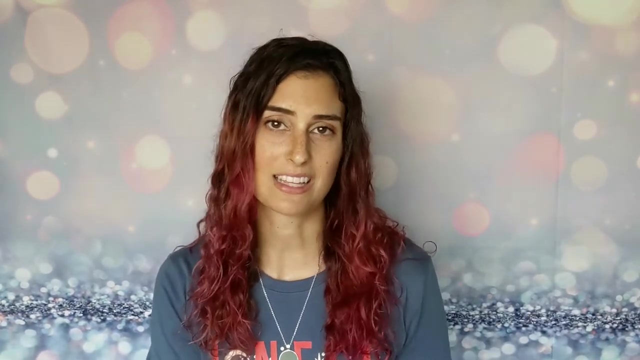 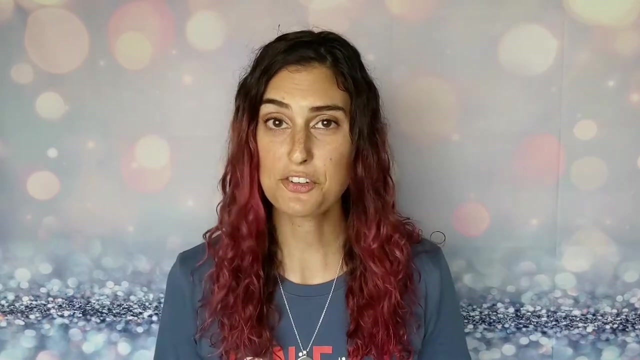 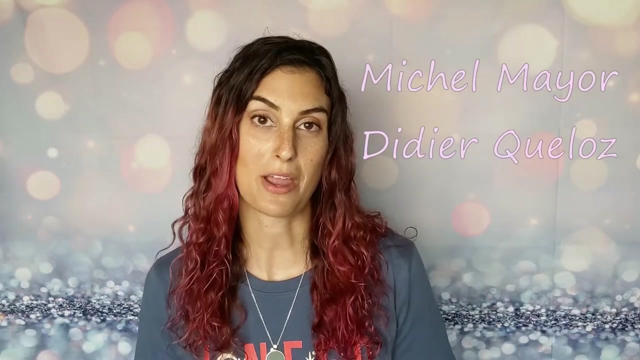 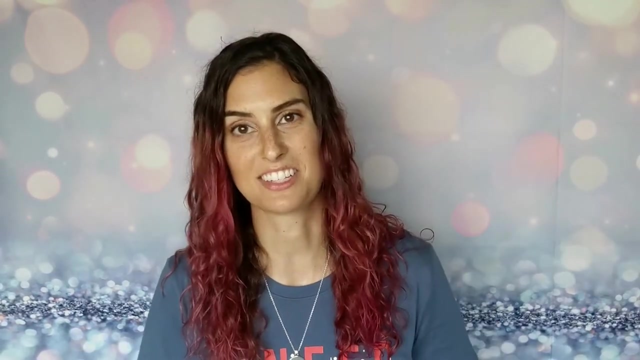 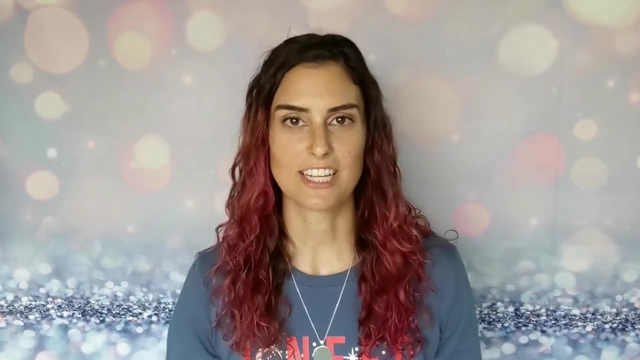 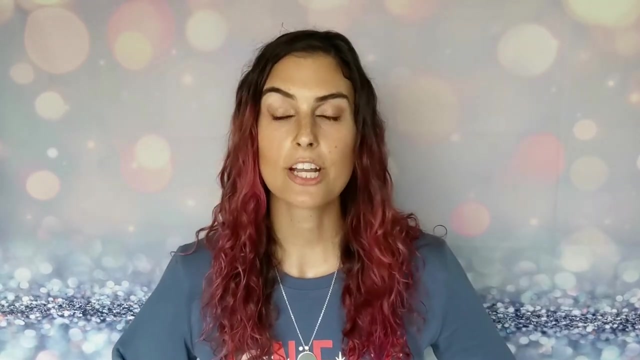 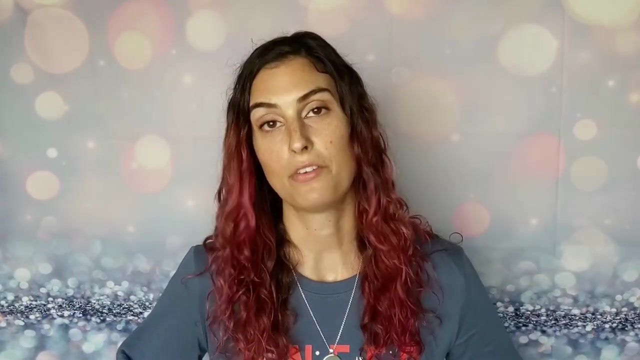 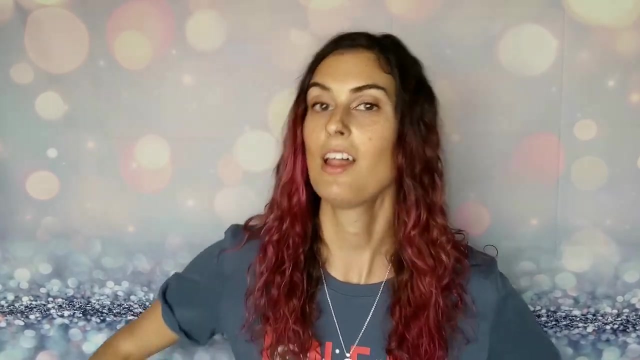 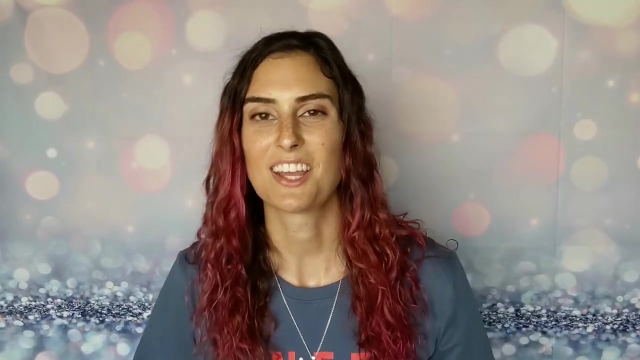 planets around a smaller star, and so the signal becomes much stronger. For an Earth-sized planet. So we are talking about radial velocity second, which means this was the second method that was used to detect exoplanets, and in fact this was the first method that was used to detect exoplanets around a sun-like star. This was a very well-known discovery around 51 Pegasus, we call it 51 Peg B, and this was published in a paper in 1995 that was led by Michel Mayor. Actually, you may have heard of this, last year in 2019 the Nobel Prize in physics was partially awarded to Michel Mayor and Didier Chouard. Didier Chouard, Nobel Prize in Physics, was awarded to Michel Mayor and Didier Chouard, for their discovery of 51 Peg B. So this was a very big deal at the time because the previous planets had been detected around pulsars, which were so different and kind of strange that we didn't really know what that said about stars like our own. So of the 476 confirmed exoplanets, 820 of those have been detected by radial velocity, which is about 90% of the total, and for a long time radial velocities was the primary method of detecting exoplanets. Until this next method that we will talk about next week, which is transits. So thank you so much for tuning in, I hope you learned something, and I hope you enjoyed, and I'll see you again next time!